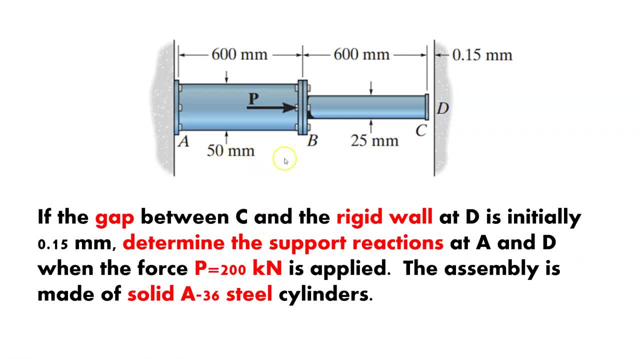 Hi, this is Professor Cummings, and I have another problem I wanted to give you for- and this will be another axial loading problem, and it is an interesting problem because it involves a couple of different concepts that are going to be added into this. 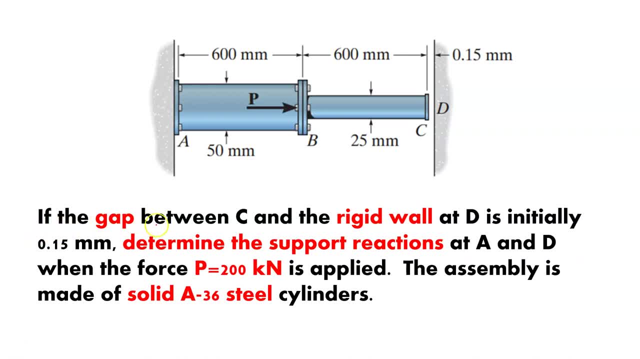 So let's read the problem here. If the gap between C and the rigid wall at D is initially 0.15 millimeters, we have C and D, so D is the wall and you have a gap of 0.15 millimeters. determine the support reactions at A and D. 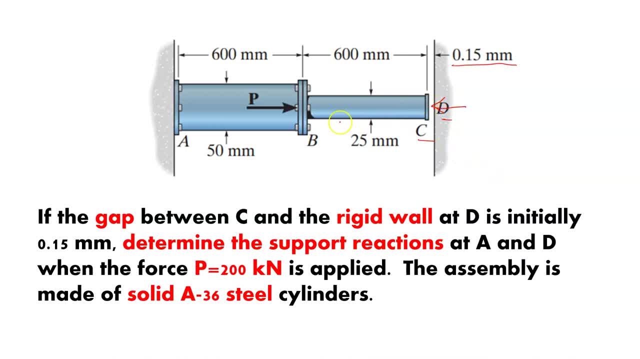 We're looking for the support reactions at the wall itself that it starts to touch and the wall that it is mounted to When the force P is equal to 200, so we have a value of 200 on this force, this applied load that's touching this joint at B. 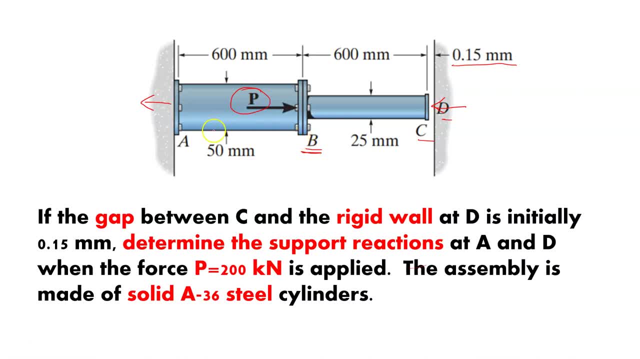 So again, first thing we want to know is: we've got two segments. We've got a segment from A to B, We've got a segment from B to C. This, all This also goes from being a determinate condition to an indeterminate condition. 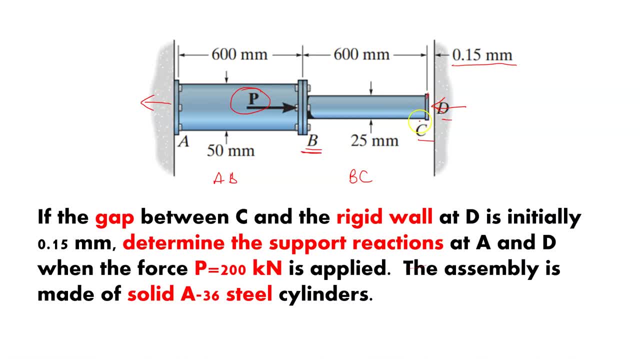 So it's a determinate condition, as it's initially set up up until it touches the wall. then it becomes indeterminate with this load applied to it. So we're going to have to come up with a way of solving this problem, keeping all these things in mind. 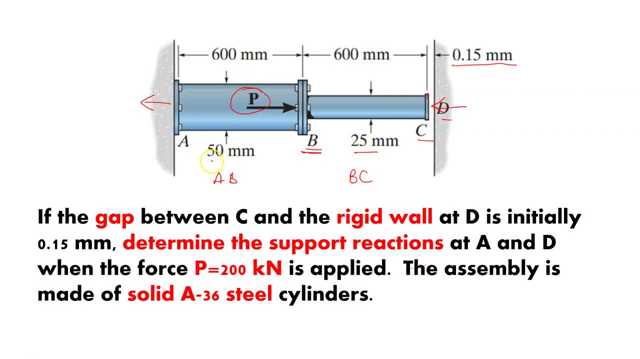 We also have a diameter for both segments and both segments have a common length And both segments have a common material. So what we know is we're going to use superposition to find the linear deformation, the total linear deformation. So that is load times length compared to the area times. Young's modulus. 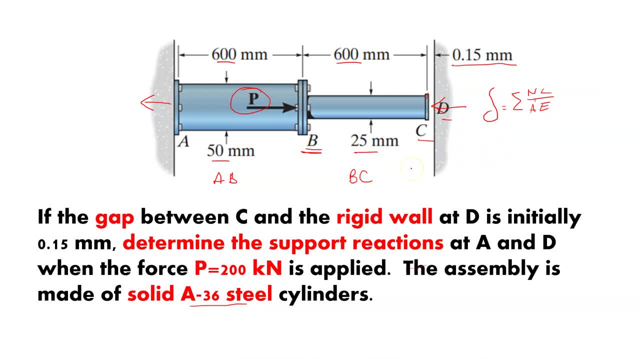 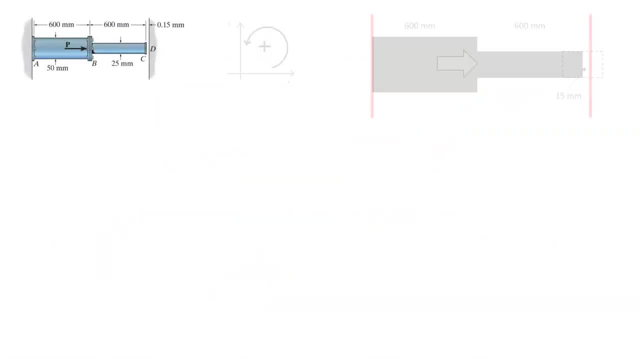 So we know that's one thing we're definitely going to end up utilizing. So let's go and set this, Let's set this problem up and we will see where we can go with this. So again, the first thing we start off with is with a coordinate system, a free body diagram. 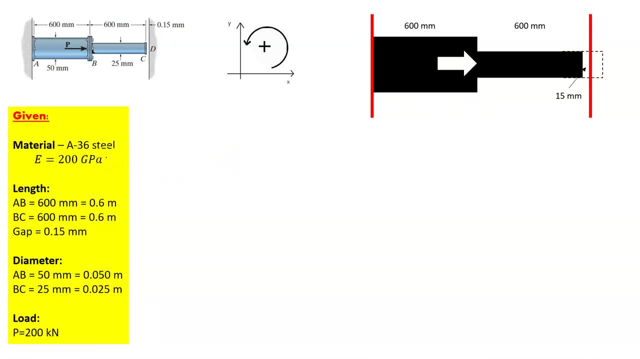 And we established everything we've been given, We've been given the material, We've been given the various lengths. Length of both segments, A, B, B C are both 600 millimeters or 0.6 meters. The diameter of A, B and B C. 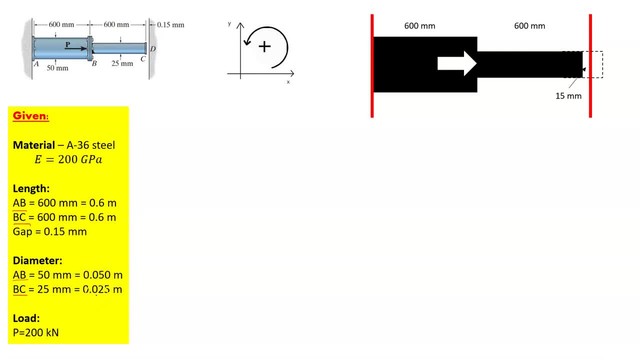 Is 0.05 meters or 0.025 meters? We got a gap of 0.15 millimeters and a applied load of 200 kilonewtons. We're being asked to find the support reactions at A and D As the load is applied. 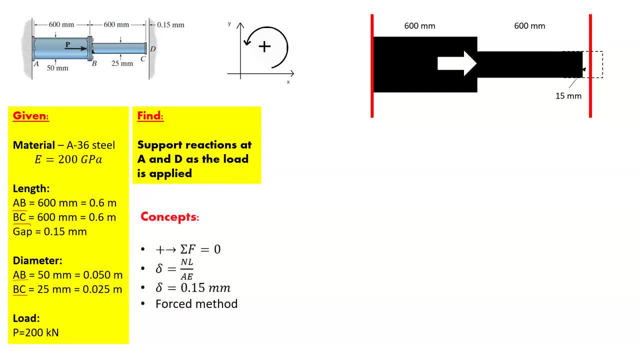 All right, so what concepts are we going to utilize here? Well, we're going to have to deal with static equilibrium. We're also going to have to look at, Uh, the deformation, linear deformation equation. we're gonna have to deal with the compatibility condition, and there are also going to have to use the force. 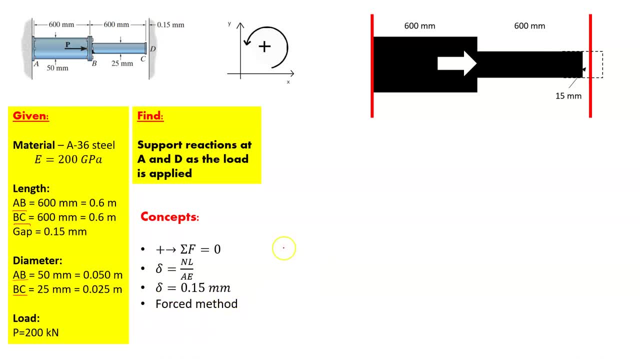 method of analysis for this particular problem. so let's solve one of the most simple things first, out of this equation, we need a cross-sectional area for both segments, since we do have, you know most of this, here we have the length, we have the Young's modulus. this wouldn't get that one. that was an easy one to solve. 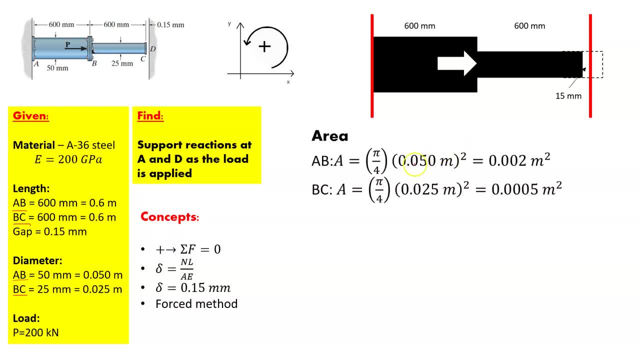 so the area of a B- you know pi over 4 times the diameter squared, is point zero zero two meters for a B and it's point zero zero five meter squared for segment BC. so the other thing that I wanted to add to my free body diagram I didn't put. 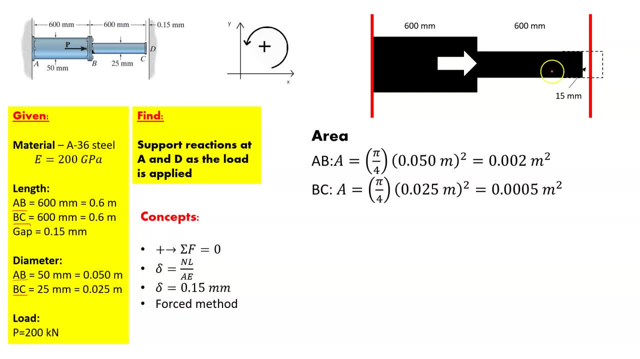 this on initially is we will have a support reaction- you both- at a and a reaction at B, but it will only happen at B as it touches the wall. so what the B is our D. excuse me, what D is actually doing is it's actually stopping or preventing this distortion. if this were to remain as a 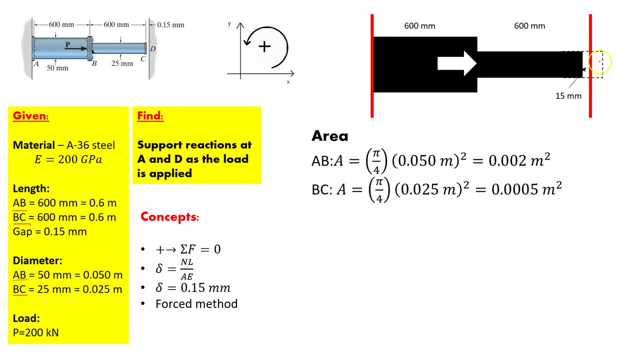 determinant condition. so really what it is is addressing this displacement that would theoretically come into play. so that's what the support reaction would look like in both cases. so we're gonna assume that it is going in the opposite. the negative action that a has is going the negative direction, resisting at D. so that means 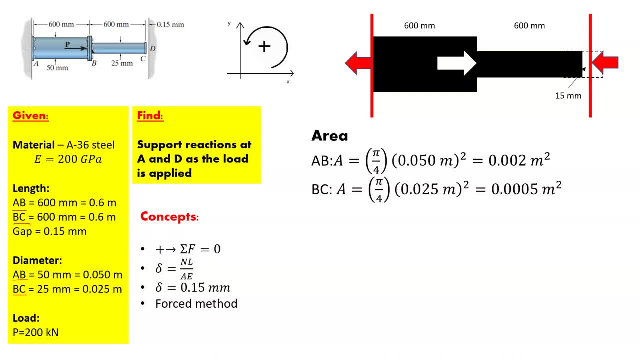 person can do it. this type of problem is start with our equilibrium equations. so I'm gonna take the sum of the forces again. go into. the right is zero. so if you look a lot what our visualization is, etiology will be 0. so what? author beside me, M is 0. so lets go into the table, come in. 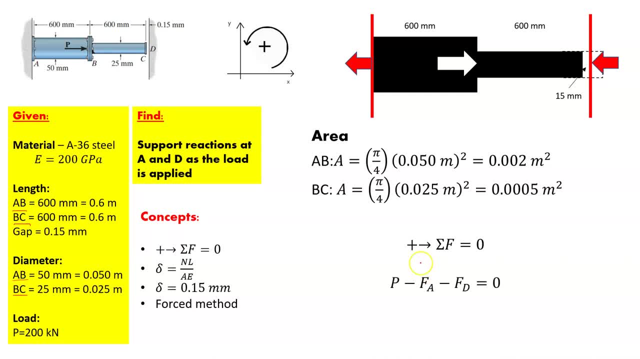 all forces are at play here. you've got the load p that's being applied, minus the reaction. it at a and the reaction at d is going to equal to zero. so that comes out that p is equal to a plus d, which is all going to still come out to 200 gigapascals. all right, so we've basically gotten the problem. 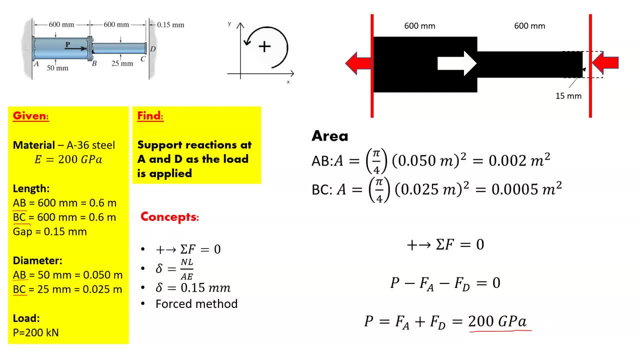 initially set up. we've got to start off with the simple things of coming with the cross-sectional area, trying to understand the logic of the problem, and came with a static equilibrium for how the forces- you know, the force, the applied forces and the support reactions are going to to interact. 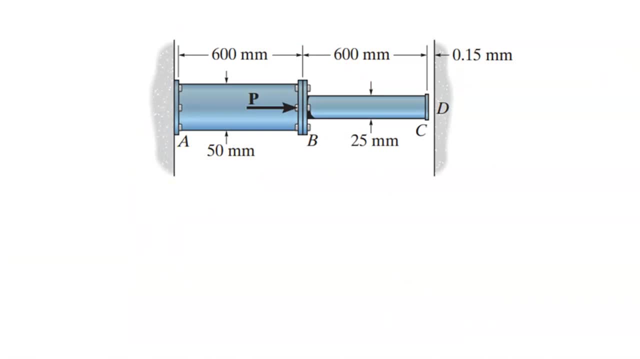 if you go back to the initial problem again and look at, try and reason through things a little bit more. so what, what can we say? we do know here. you know kind of review things. we've got a 200 kilonewton load and it's going to force section a b into tension. 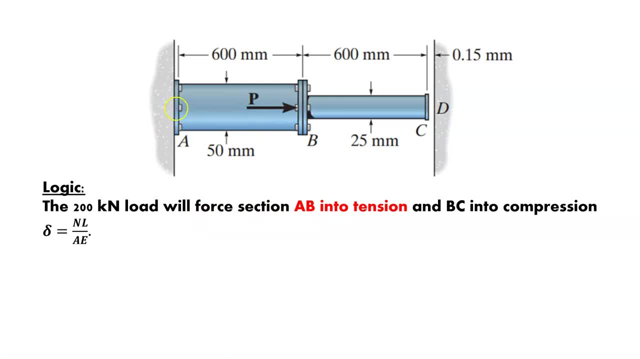 you know it's going to pull in one direction to have an equal and opposite reaction in the other right, and b b, c will be in a state of compression as it forces it into the wall. so we get a reaction going in that direction there. so we know that's going to happen for sure. 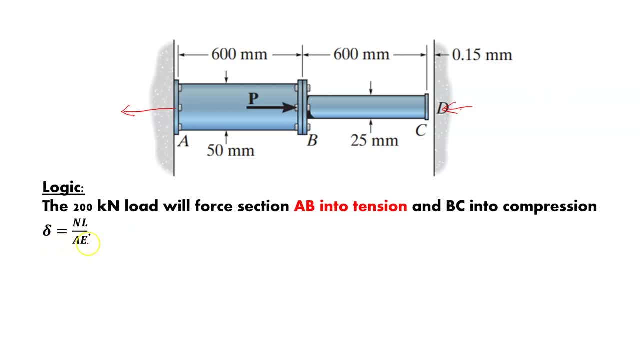 we also know that we're going to need this, our displacement equation, both addressing what's going on at a, b as well at- but it won't really happen quite at d until it meets the wall. so that's where this compatibility condition takes place. so it's going to displace this amount and nothing more but that. 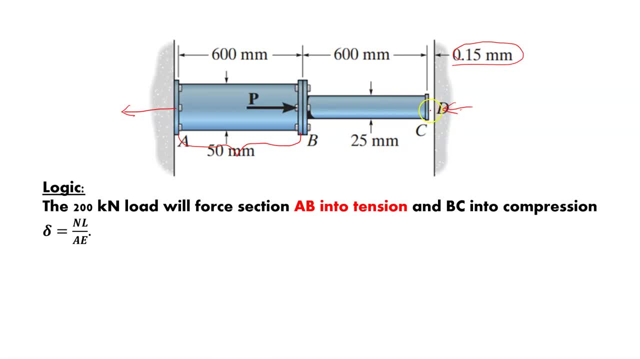 load is going to exceed, potentially exceed what, what would happen at that reaction of b? and that's, it's the, the dashed line, phantom line, one through d. so what d is doing is it's basically compensating for this, this displacement, to match that compatibility condition. so the wall d will create a reaction force, so the net displacement. 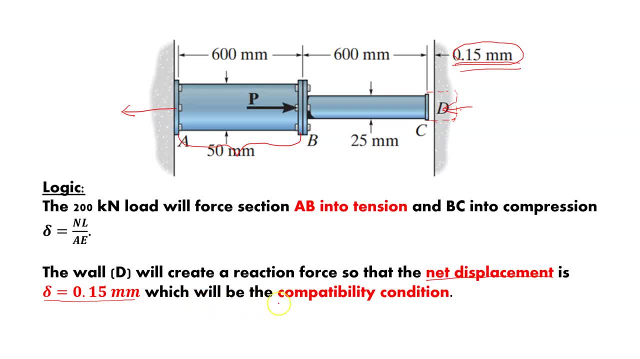 is basically just the gap, which will be the compatibility condition between the curve and the wall that we need. so what we're looking at for that total deformation, which is only going to be 0.15, it's only going to fill the gap and then it's going to stop due to. 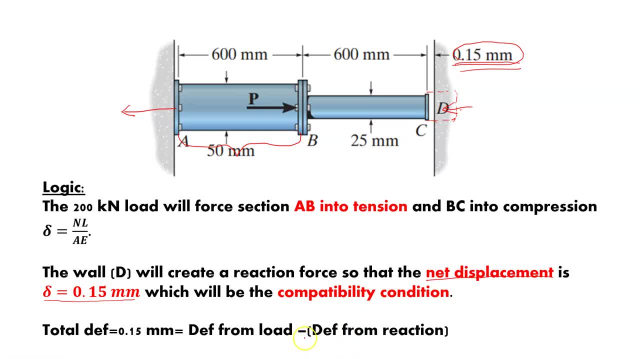 the reaction of the wall. it's going to be the deformation from this load which is going to push it to the wall, minus the deformation which is caused on this reaction. and keep in mind this reaction is going to be to both segment, BC and AB. so this is going to be the more challenging part of 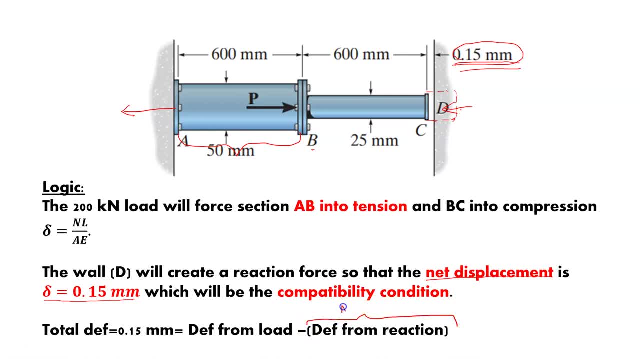 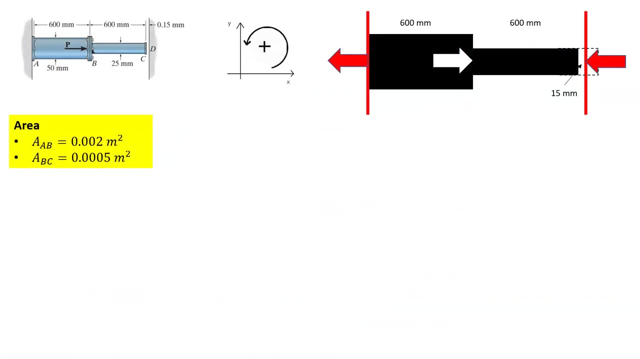 the problem. so this is going to be applied to a, B and B C. you know, in that, in that reaction, even though the deformation from the load is only going to affect a B, all right, so let's go back to our problem. again. we calculated our areas. we also know what the static equilibrium is gonna be, based on our 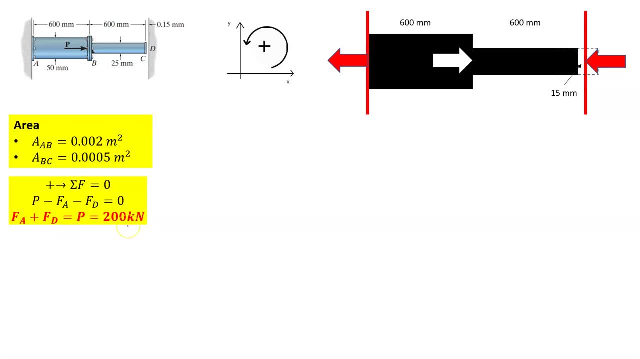 reaction loads and our applied loads, there will be 200 kilonewtons. we also know that our compatibility is 0.15 millimeters and it's the displacement of a be minus. this os understanding of. frankly, this is also the state happiness side. pero we're not true. there is one little contributionا of plastic vedere. 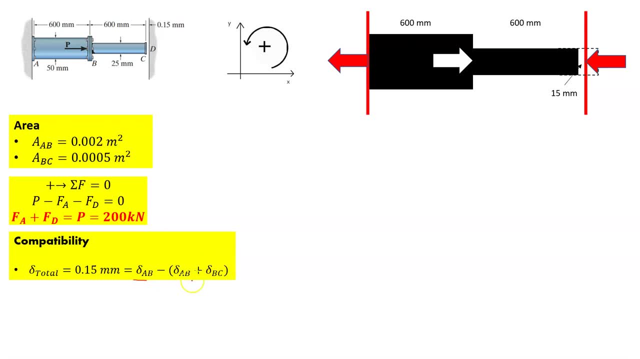 the reaction due to D, the displacement that's going to be imposed on both segments. so superposition, that is to utilize that that term, superposition. so let's figure out what is going on at a, B first, based on that load. so if you look at the load, the deformation due to load P, here we've got the load of a B times. 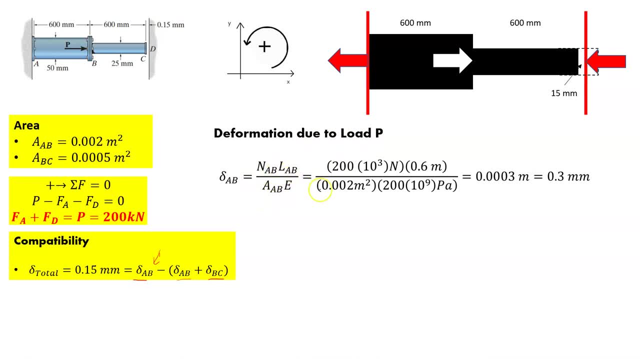 the length of a B over the area of a B times Young's modulus, so that's the 200 kilonewtons K is just 10 to the third and 0.6 meters length. and then this cross-sectional area, 0.002 meters squared and 200 gigapascals, or 10 to the. 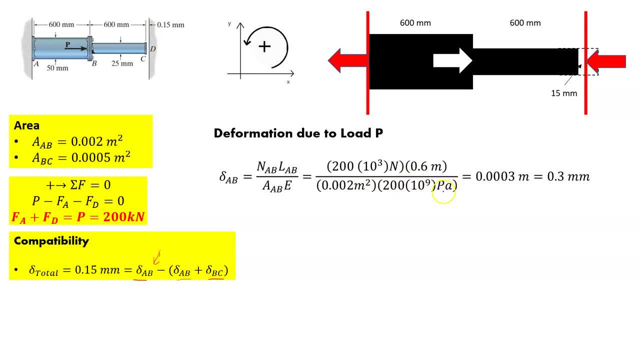 ninth gigapascals. if you notice, a Pascal is just the Newton per meter squared, so this cancels. you can always check your units making sure that they come out correctly and you end up with nothing but meters for your displacement, which is point zero zero three meters or point three millimeters? so as you can see, if just on, 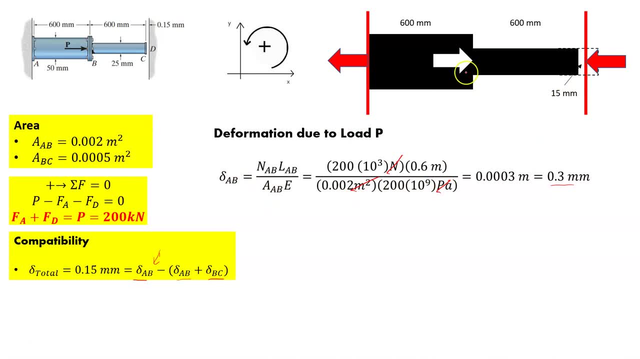 that load alone, that 200, 200 kilonewton load you're, you're moving it. you would normally displace this twice as much as that gap. you go 15 millimeters and then without that wall there you would actually take it out to point three. 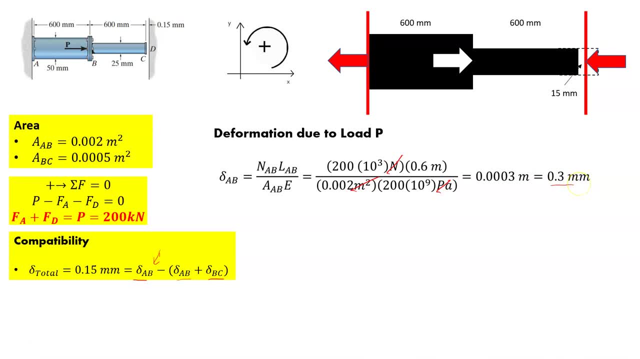 millimeters, so the wall is stopping what's going on, and that means that a- B is going to get a bigger reaction because of that. so now consider what deformation has taken place due to that reaction at D. we have to do is look at both segments- a B and B C- and we're looking at what that reaction to the D is. 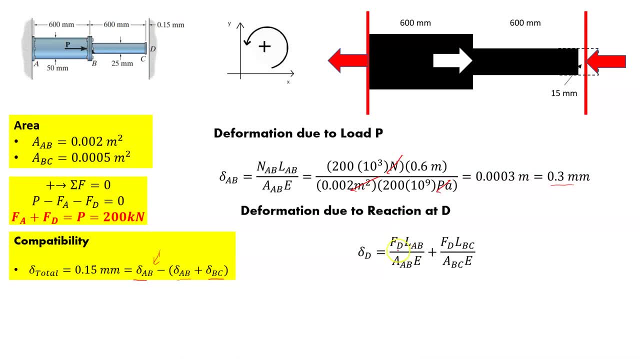 So this is the reaction force at D. Now we're looking at the length of AB, we're looking at the area of AB and Young's modulus. same going on at BC: the length of BC, the area of BC and Young's modulus. 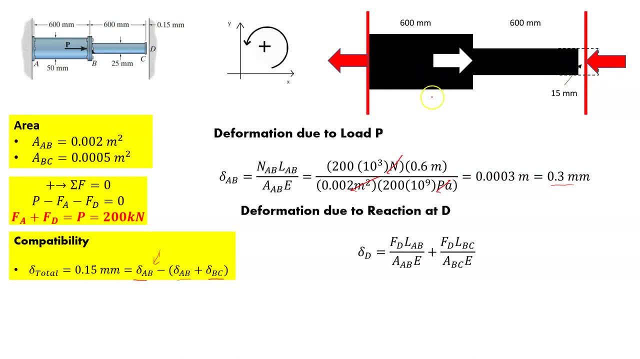 So keep in mind that reaction force is going through the entire member. That's why we're able to use superposition to understand that. So we've got a reaction due to the load that only gets applied to AB and a reaction due to the load at the wall that applies to both AB and BC. 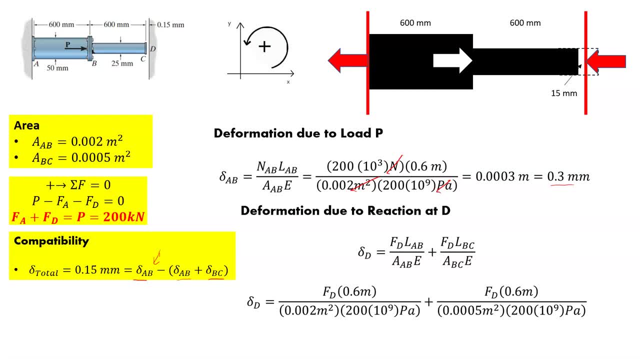 So we plug in our numbers and we still don't know what that reaction is. so we just represent it as F of D. So we've got the length, the cross-sectional area, .002 meters, squared at 200 gigapascals, which is our Young's modulus. and for BC, the same length, a different. 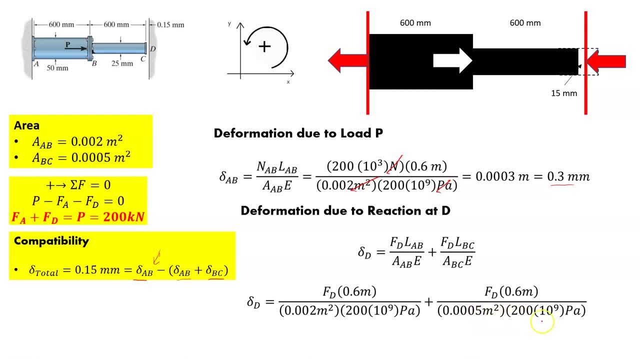 cross-sectional area: .0005 meters squared, same Young's modulus. So if we reduce this we end up with 1.5 times 10 to the 9th F of D, plus 6.0 times 10 to. 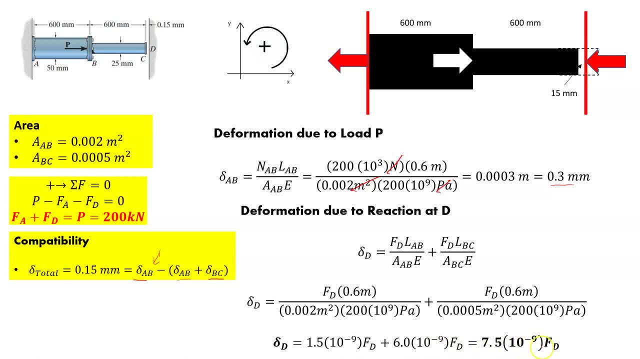 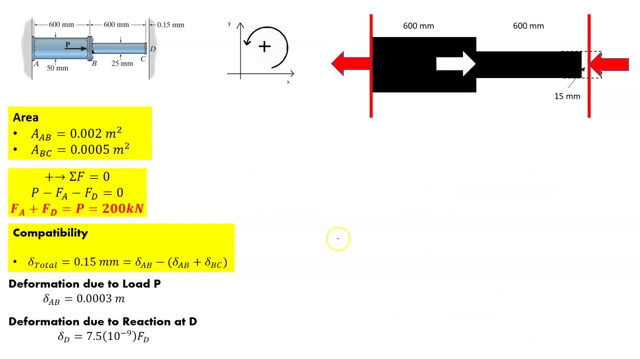 the 9th F of D, Which just comes out to 7.5 times 10 to the 9th F of D. So we still don't know what F of D is. We have a function to describe the displacement that D is going to impose. 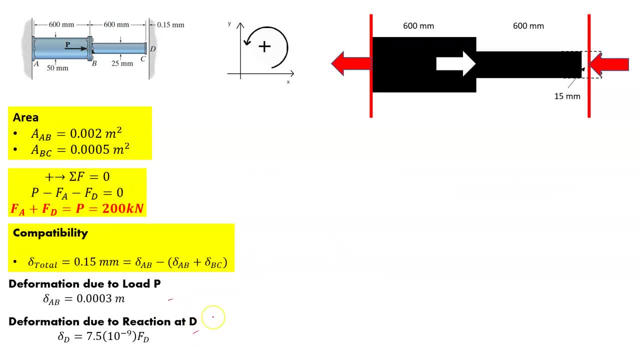 So we've got our findings here, So now we also can take into account that compatibility equation. So the compatibility equation- this is why that's so important- it's .15 millimeters and again, we know that that compatibility condition is basically the difference between: 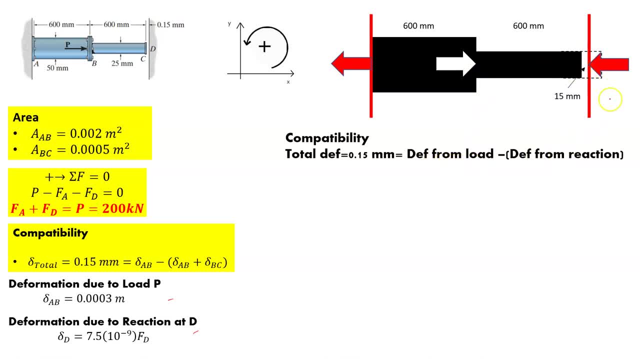 how much this is going to go in one direction minus the force reaction from the other direction. We know that's going to come out at .00015 meters. just put this into meters just to make it easier on myself, and that's the way this equation looks. 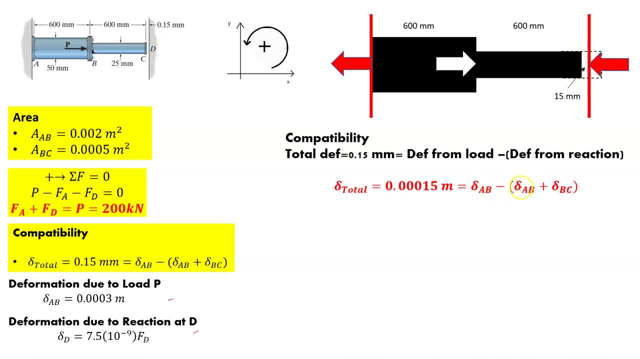 So it's the displacement of AB minus the force reaction from the other direction, The displacement of AB minus the displacement, the quantity of the displacement of AB plus the displacement of BC. So both segments of that rod is equal to our compatibility condition. So plug in its values. you can remember we had this reaction force at D and we end up. 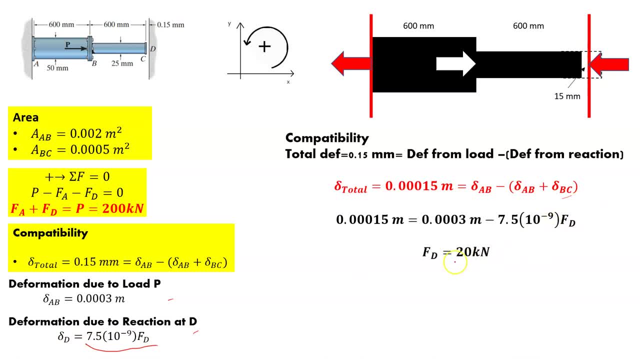 with .00015.. So we've got 20 kilonewtons as the reaction force at D. Now keep in mind, we've also got this to worry about our compatibility equation. So we know the force at D and we know that the force that is being applied is 200 kilonewtons.